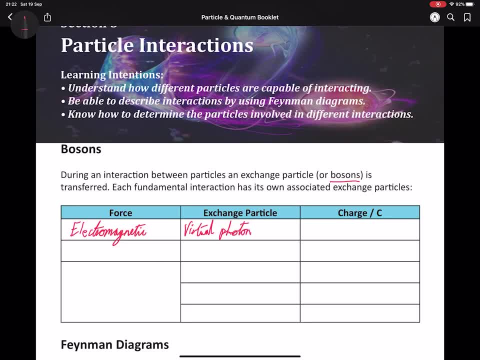 electromagnetic force, or the electrostatic force as it's often known, we have a virtual photon shown as a gamma symbol. Now, this is just a photon that exists for an incredibly short amount of time, hence the word virtual. And as it's a photon, it does not carry a. 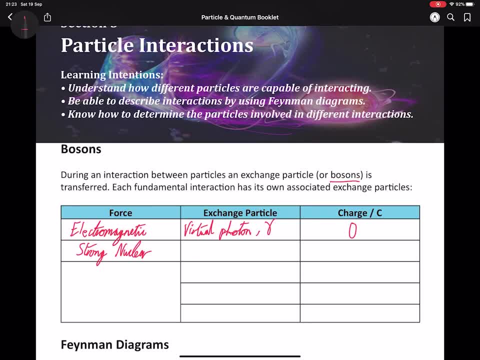 charge. Now, the strong nuclear force, as we know, binds the nucleus together. So it's given the very easy-to-remember name gluon, given a symbol, lowercase g, And again this has a charge of zero coulombs. It's just a binding force, not transferring any real changes. 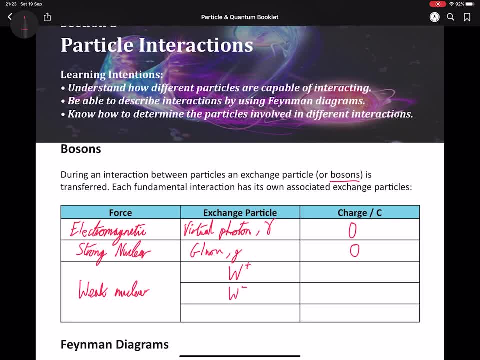 Now the weak nuclear force is different. It has three different versions. The W+, as the symbol denotes, transfers a bond. The W- is a positive charge, So 1.6 times 10 to the minus 19 coulombs, Whereas W- will. 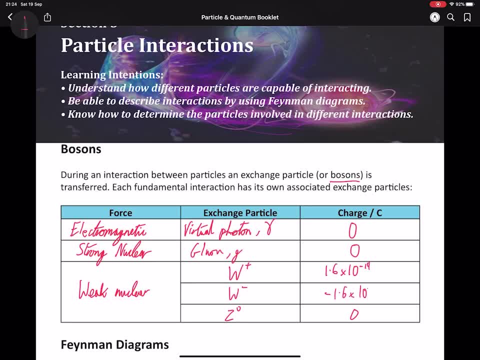 transfer minus 1.6 times 10 to the minus 19 coulombs. Now Z0 is an alternative, one that transfers no charge through the weak interaction but is rarely going to come up. It is mainly just a referential particle. 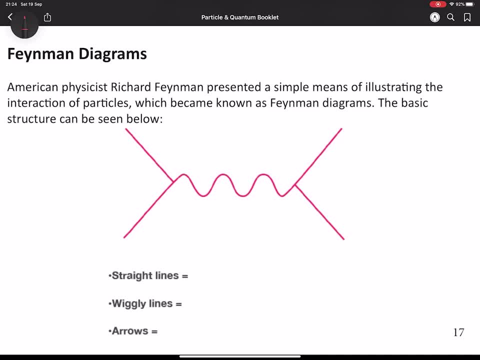 Now, in order to show interactions clearly without vast amounts of mathematics, what we use is a Feynman diagram, Designed by Richard Feynman. these were meant to simplify interactions and have a few basic rules that we follow. Now be aware, some of these rules are slightly 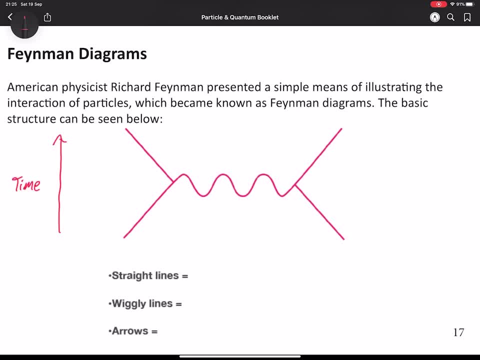 different when different people do this. So the rules we're following here are the AQA-focused rules. So these diagrams are red from the bottom to the top. That represents the flow of time. Now these angled lines moving in, these straight lines, they represent the particles that are. 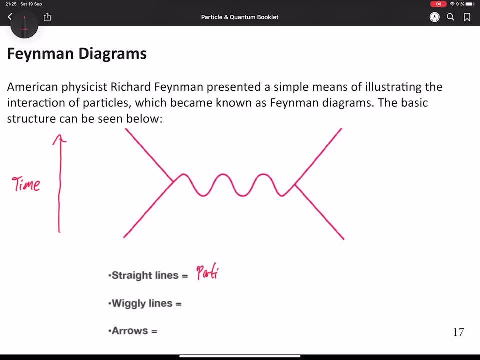 going to interact. At an angle, you might think that they're showing them moving closer to each other before they interact, But that's not the case. It's showing them moving to interact in terms of time. So below the squiggly line in the middle. 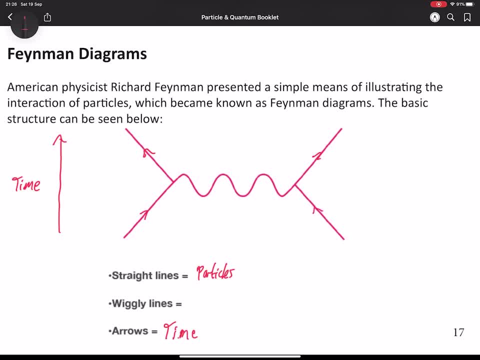 we're talking about an interaction about to happen and, above that point, the interaction having happened, So time is represented in the diagram itself with these arrows on each particle line. Now that doesn't really matter too hugely for us, But in some versions of the diagram it's. 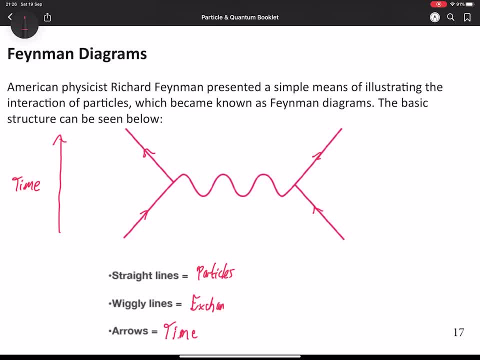 better to keep that in mind. In fact, if you're looking at some of the other diagrams, you might see that there's some versions that are not AQA based. inverted arrows might represent an antiparticle, so be aware of that. The wiggly line in the middle is your exchange particle and it's red from left. 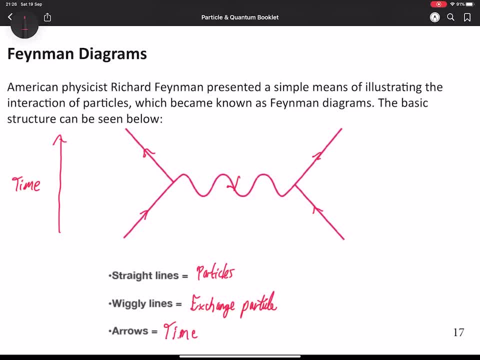 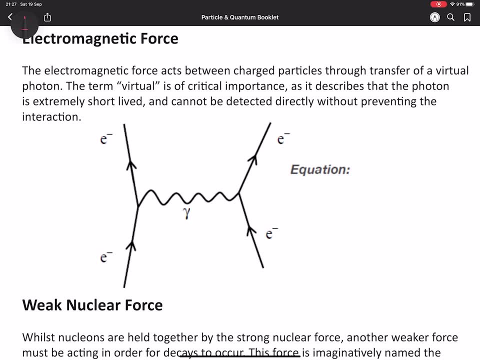 to right, so we can add an arrow here, but it's not necessarily required. So looking at some examples for these, you're expected to be able to translate from diagram to equation and vice versa. The electromagnetic force is the easiest. not much happens. We get an exchange, as shown here by the gamma symbol of the virtual 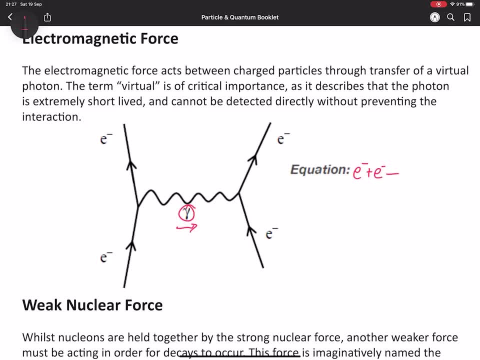 photon, and in this case all we're seeing is two electrons interact, transfer virtual photon and we end up with two electrons that have now repelled. This has no symbolic form in an equation, so the equation is relatively meaningless. The weak nuclear force, however. 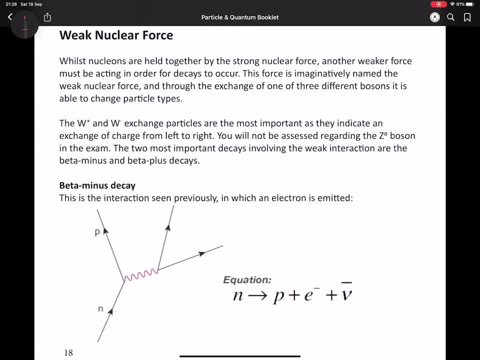 has some key examples that are far more important to be able to transfer. So in this example here we're going to see some W plus or W minus particles transferred. So for beta minus to begin with, this is your traditional beta decay. Now we start with our. 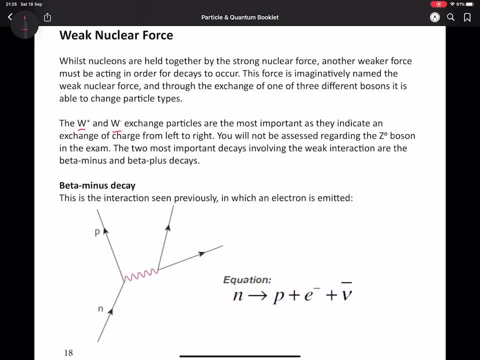 electron, which turns into a proton. Note that the large particles like these are on one side of the diagram. This will have more meaning later in the booklet. Now we end up with these two tiny particles as well: the electron and the antineutrino. 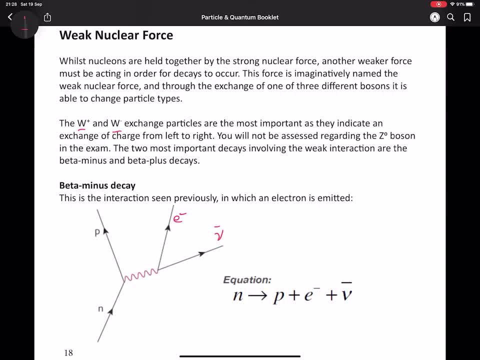 Both of these can be represented at the top right here. It doesn't matter which arrow is which, because they're both above the central point. They're both a result, a product of this interaction. Now, it's a W for the exchange of a charge, and it has to be W minus in this case. 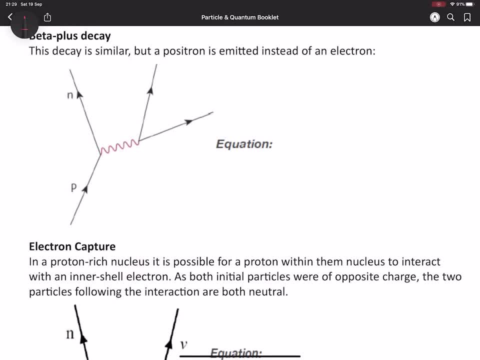 Reading from bottom to top, we can follow the charge. Now that is better represented and explained with beta plus decay. Now this is similar to beta minus decay. so instead of ending up with an electron, we're going to end up with a positron. So in this case, the proton is caused to decay into a neutron. 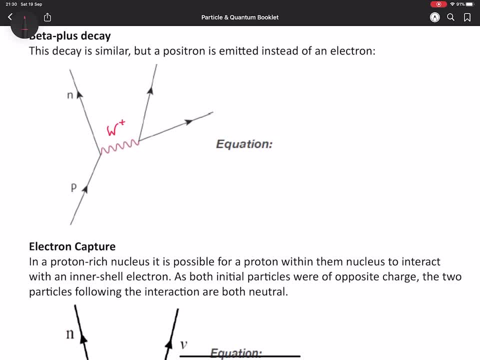 If we follow the charge, the proton has lost its positive charge, so that is released as a W plus boson That needs to form itself into a long-term particle, so it becomes a positron And, as we know, when an electron-type particle is formed, a neutrino-type is formed as well. 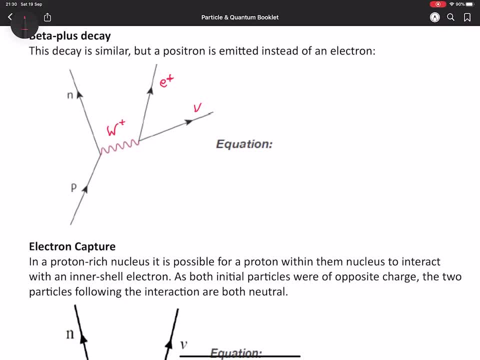 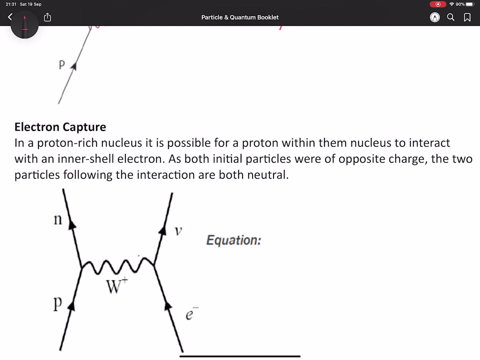 And in this case, because the positron is an antiparticle, we end up with a particle, neutrino. So again, this is exactly the same structure as beta minus decay, our traditional beta decay, but we've changed our quantum values. So we can see that the electron capture is a unique interaction, an example of a weak interaction. 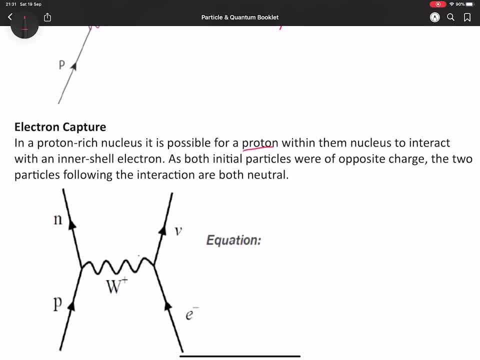 that we need to know about. So this is where a proton in the nucleus manages to pull in an inner shell electron and convert itself into a neutron. So we can see here that we actually end up with two particles at the beginning. A W plus transmits from the nucleus to the electron. 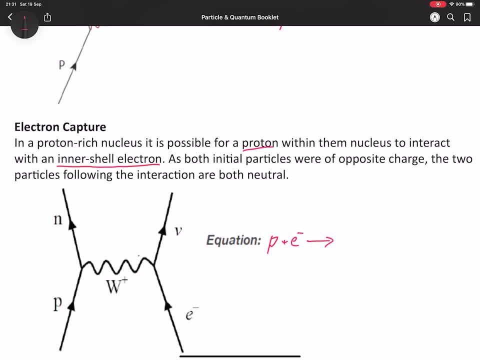 So we can see here that we actually end up with two particles. at the beginning, A W plus transmits from left to right, which means the proton loses its charge, becomes a neutron, and the positive W plus cancels the negative of the electron, leaving you with a neutrino.